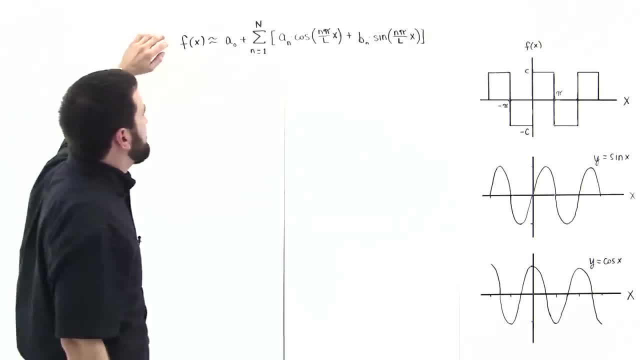 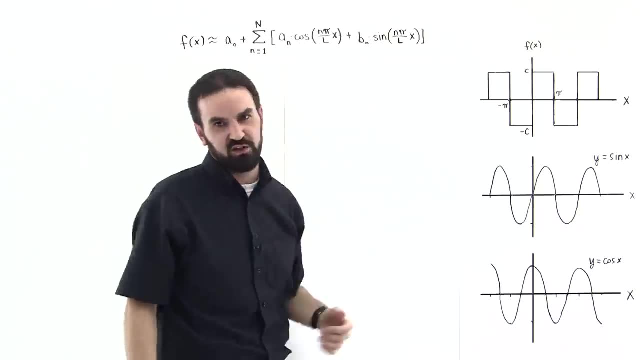 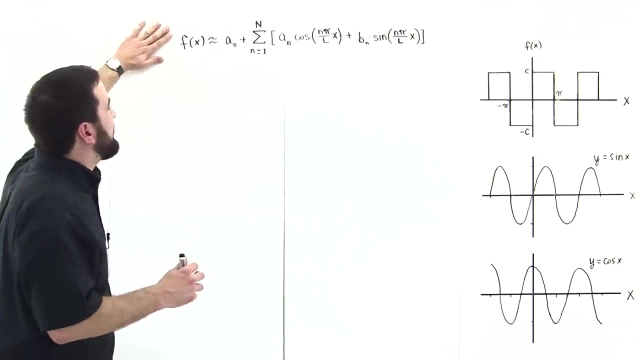 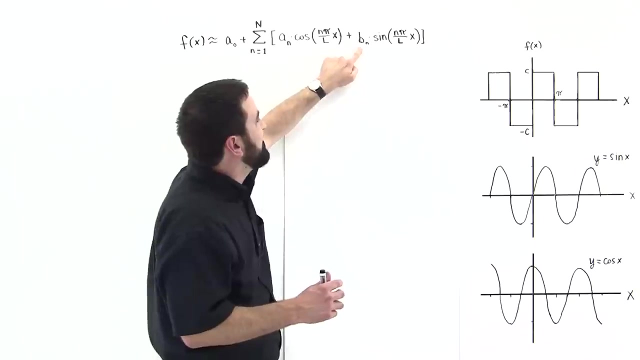 this function could be approximated by some constant plus a sum of cosine and sine functions, A combination of cosine and sine functions, And that any function could be modeled with this, Given that you could find the coefficients this a sub n and this b sub n to match it up. right To make things, 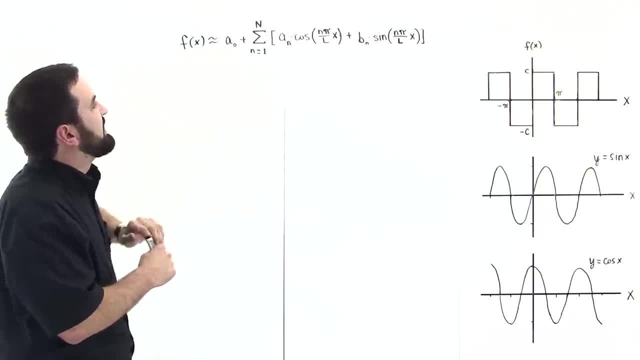 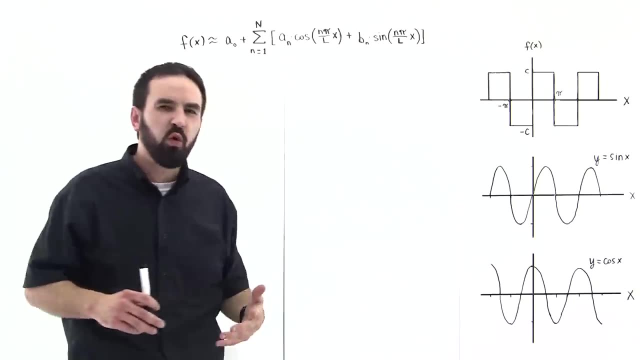 fit. Okay. And also this constant here, a sub 0.. Okay, so we look at these. and let's look at this sine function. let's look at this cosine function. Which one of these do we think is going to do a better job of modeling this function? Which one do you think? 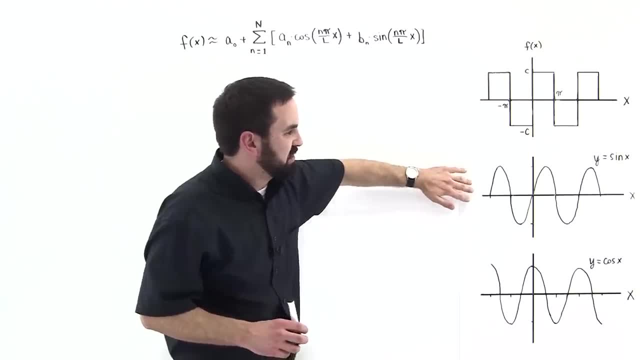 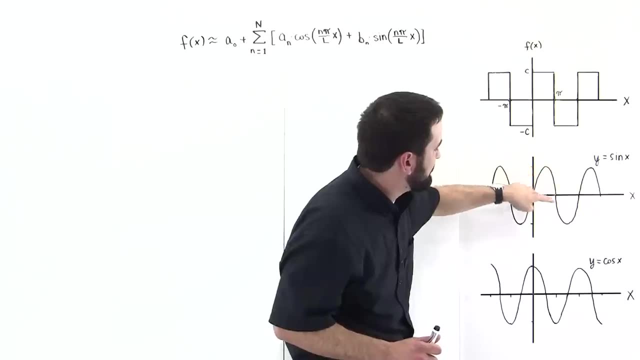 will do a better job. Well, I would guess that the sinusoidal function would do a better job, The sine function. that is Because it approximately matches the period. Well, it exactly matches the period. Look, this one has come from negative pi and negative. 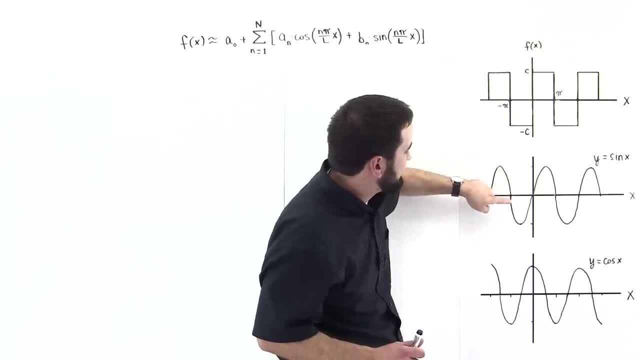 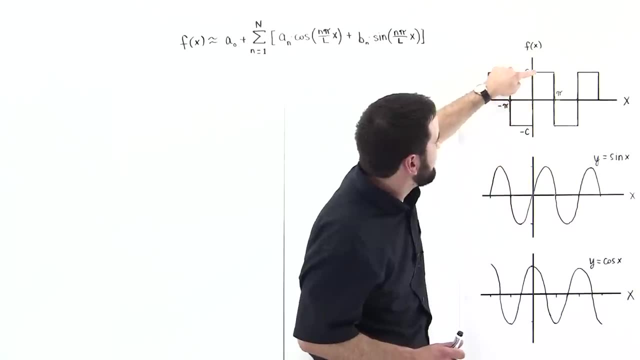 pi is coming down and over And negative pi- this is coming down and over. And then from zero- this is zero- to pi it's coming up and over And then this is coming up and over. So if we superimpose this on top of this, it would do. 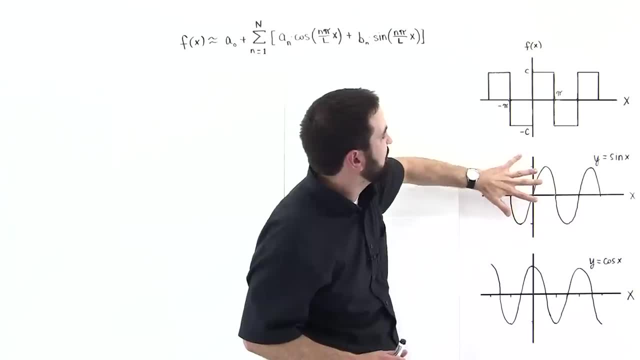 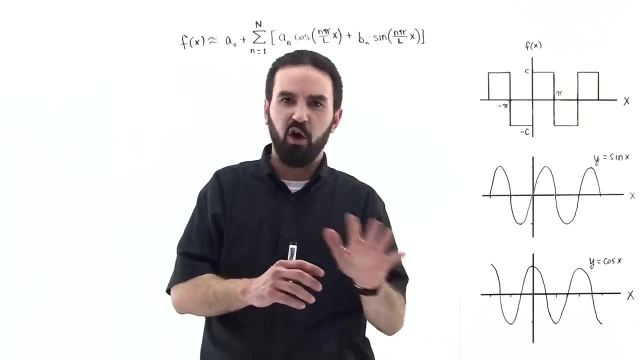 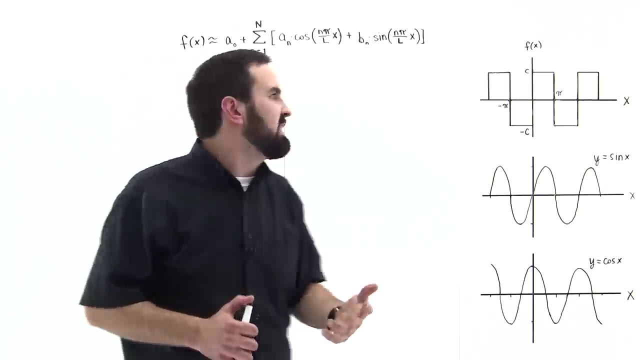 like this. So this sine function is more is a better approximation to this than this cosine function is. The cosine is off right. It's out of phase with the function that we're trying to model. So if we were using these terms here, 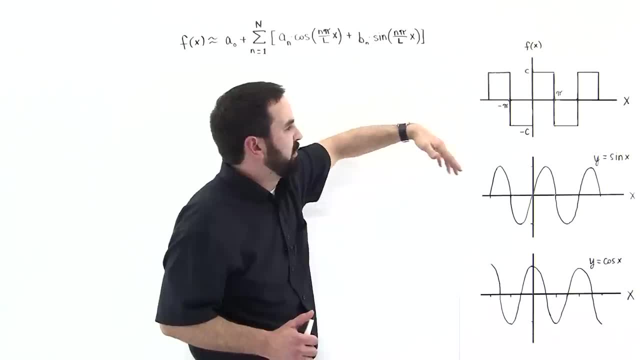 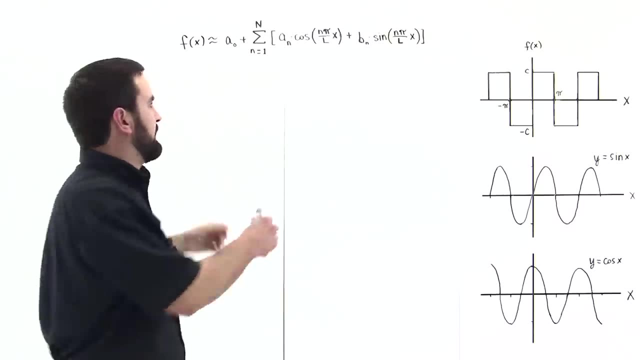 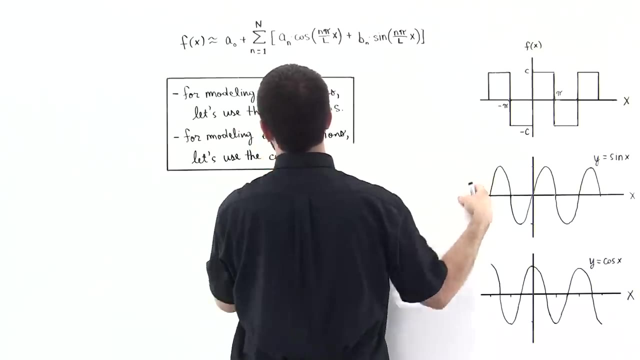 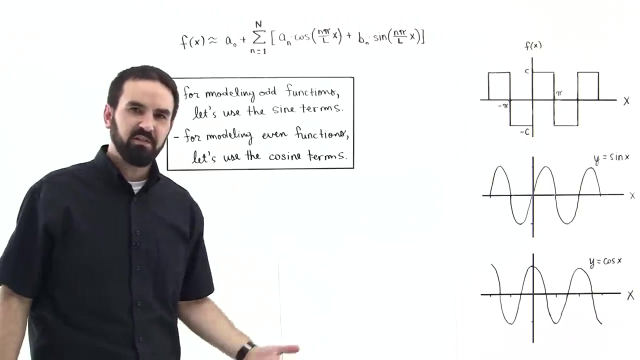 in our mathematical model that we're used to model this, these cosine terms would be working against this. So we conclude the following: When we use, when we use for modeling odd functions, let's use the sine terms, The sine function, And for modeling even functions, let's use the cosine. 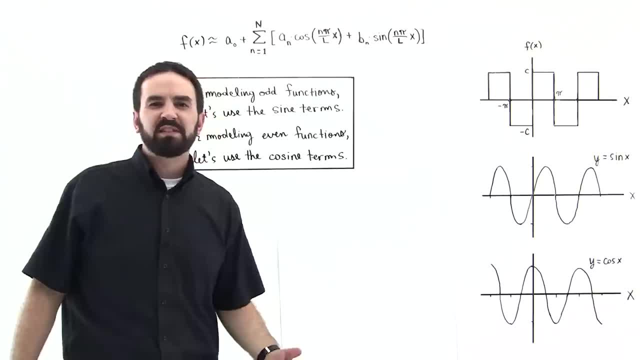 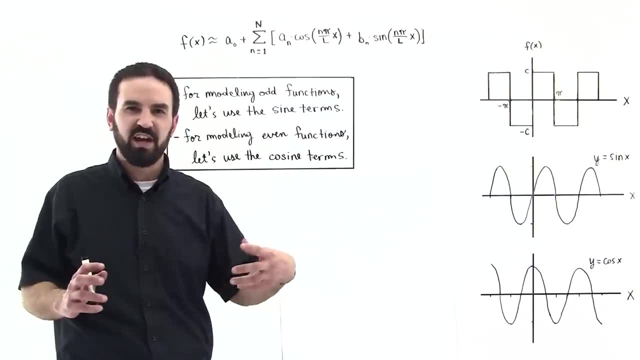 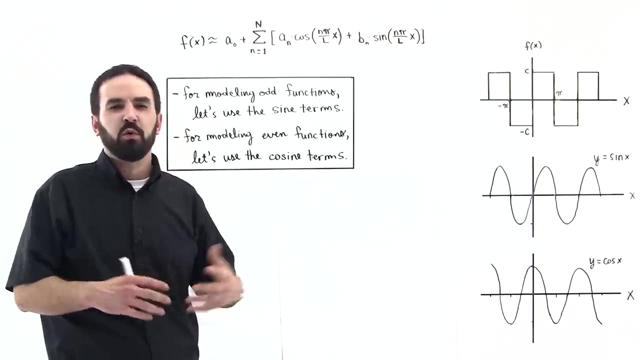 Cosine function Make sense. Now there will be some functions. remember, I said any function. So there will be some functions where you will use a combination of cosine and sine terms, But for this one, because it's strictly an odd function, you will only use the sine terms to model this function. 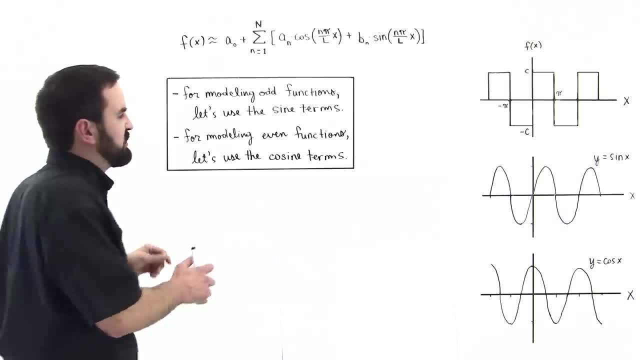 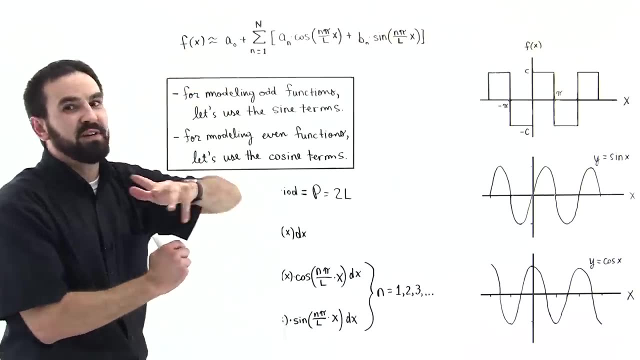 And in the next tutorial, part two of this series, we will show that that's true. Okay, here we go. So let's take a look. The next, the real, the hard part. the brilliance of Joseph Fourier was identifying what these constants would be. And here they are. 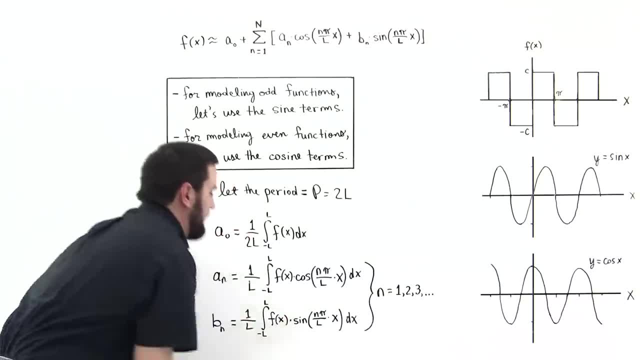 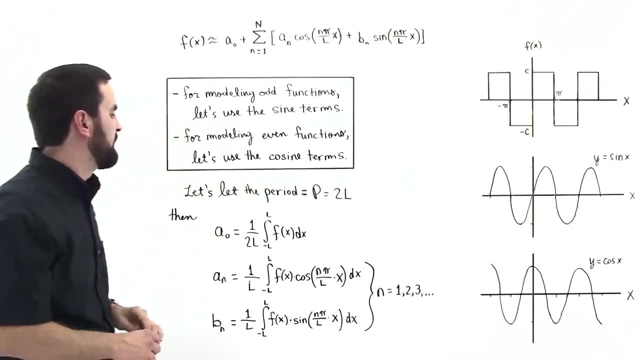 So Joseph Fourier in the early 1800's said: what if we let the period be equal to 2L? Then these things would be true. Okay, so the proof is in your book. We will just do. we are going to do an application. 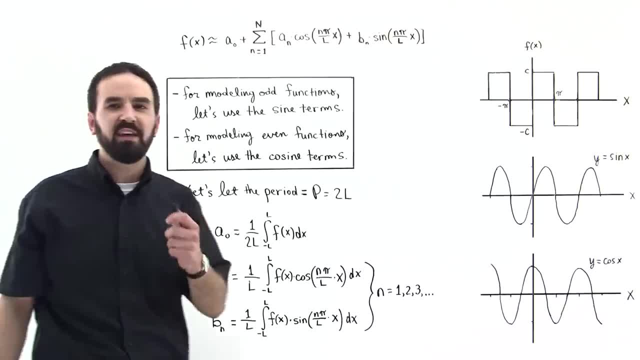 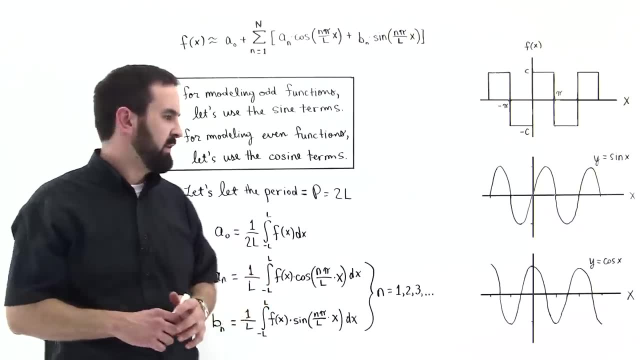 and zip through this kind of quickly. But the application- I've done this, I've been in your place, I've learned this before And the application is where you really see it come together when you graph it And you see how the what will happen when you graph it is the function will come up. 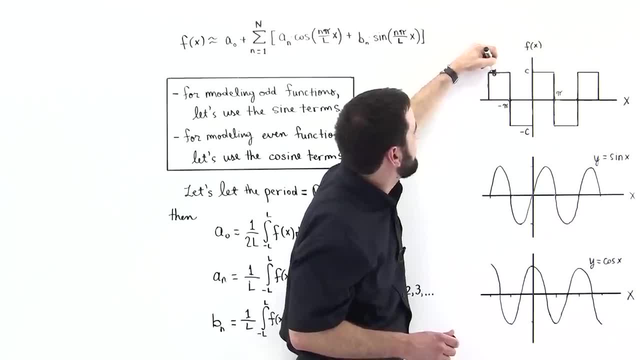 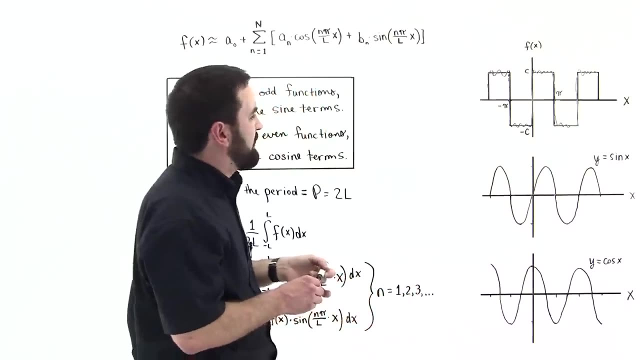 you will watch it on your calculator and it will come up and it will do this number And then, when it gets to here, it will come, it will come, it will zip down like this and it will do this like that. So and the more terms you add, if you added. 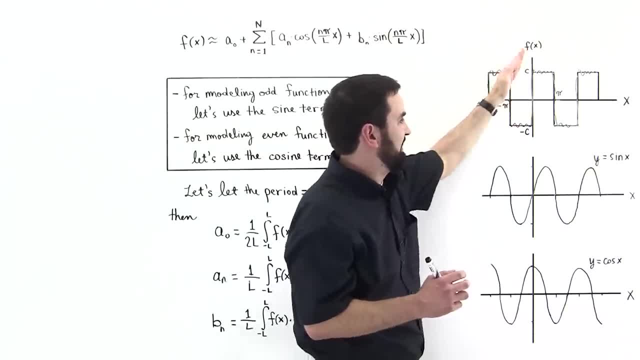 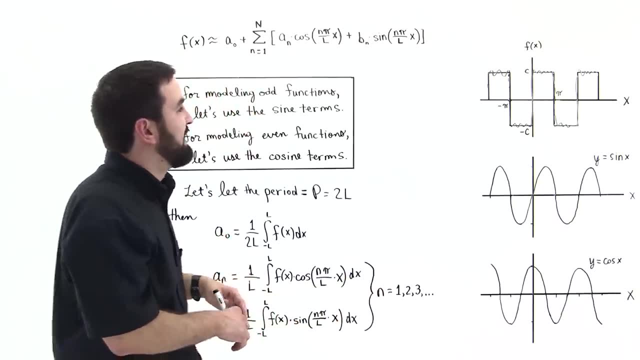 an infinite amount of terms, then it would match this thing exactly. But of course no one can add an infinite amount of terms because infinity is not a reachable thing. but we can add a lot, And so these squiggly lines will get the humps will get smaller and smaller and smaller. 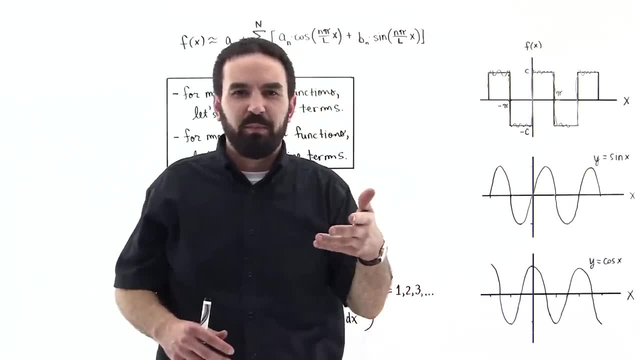 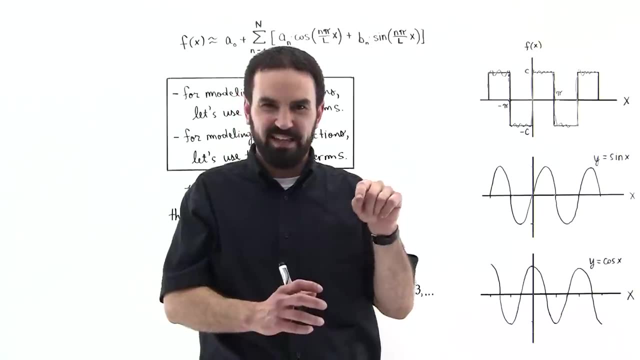 until it looks like you can't see it with the naked eye, You have to zoom down. you know, with your zoom function on your calculator you have to zoom down really tight to see the wiggling, the squiggling lines. Okay, so you see that. this for a0. 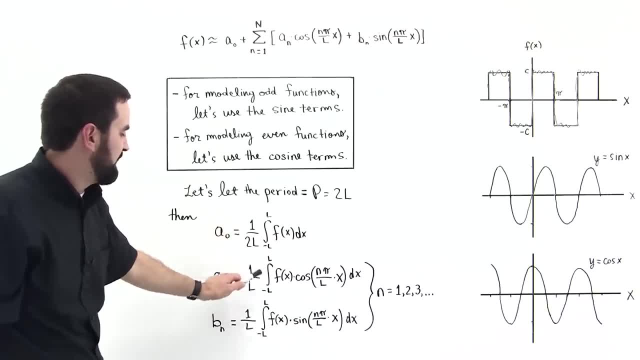 it goes from negative L to L. They are all integrating from negative L to L. So half the period right, Half the period to the positive of the other period. But notice, of the same period, it's all one period. Notice something: that this thing goes from negative L to L. 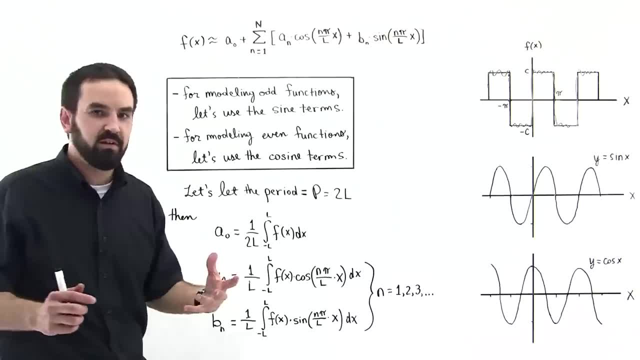 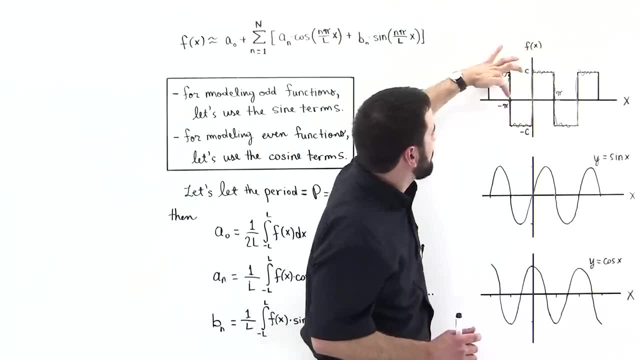 so that's one wavelength, isn't it? That's one period, Right, Because this one goes the period it goes from negative pi. one cycle is this is one cycle. Boom, boom, boom, boom, boom. That's one cycle, right. 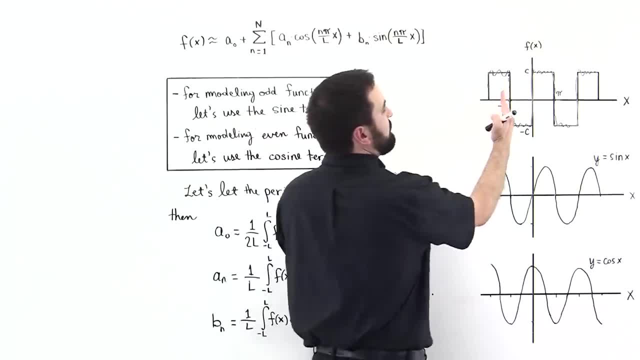 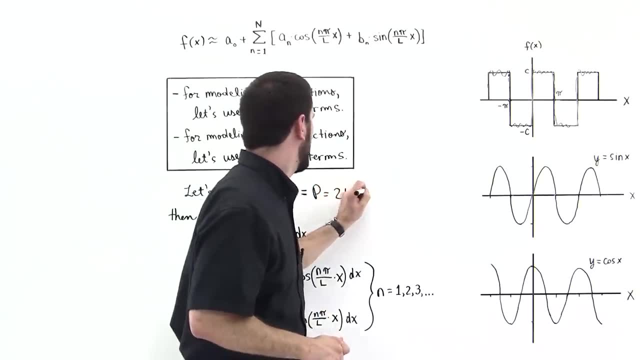 From negative pi to pi. So what's the total period? It moves over by pi and then pi again, so the period is 2 pi. So the period is equal to 2 pi, And so solving for L, L is equal to 2 pi. 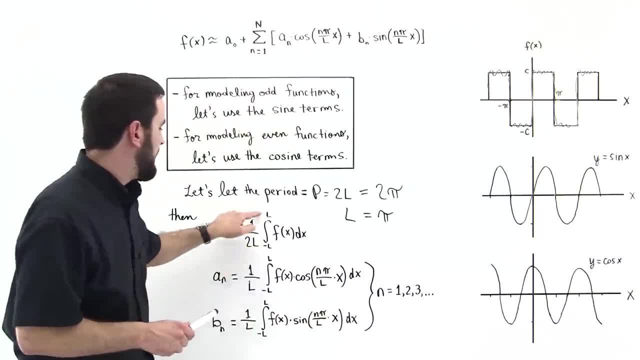 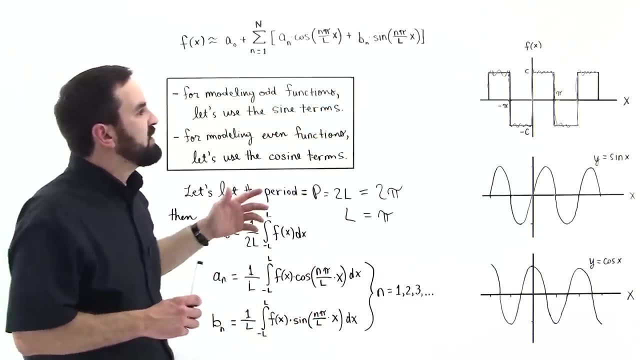 So we would integrate from negative pi to pi And then this f of x. here is the function itself that you're trying to model. But notice that this function we can't just integrate. we can't. it's not a continuous function, it's a step function. 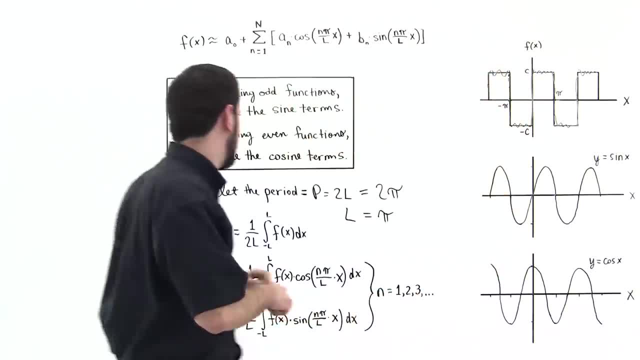 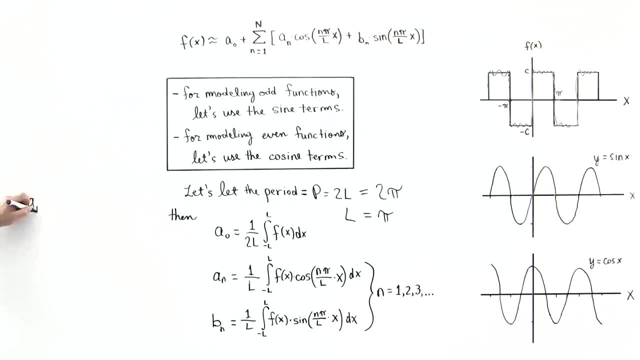 So we can't integrate continuously from here to here, so we have to break it up into pieces. So I'm going to write f of x. I'm going to write a0 right here. Step out the way here. a0 will be equal to 1 over L. L is. 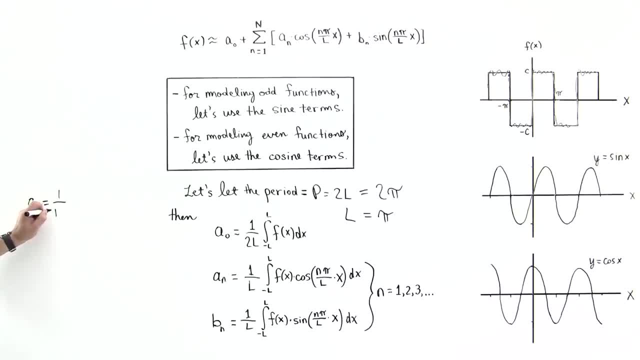 equal to pi, 1 over pi, 1 over 2 pi. Yep, 2 times L, L is pi. Okay, 2 times. open bracket the integral from negative pi to pi. and we're going to. well, no, pardon me, we're going to go from. 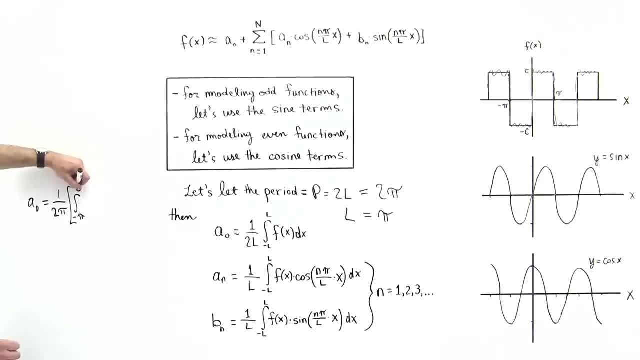 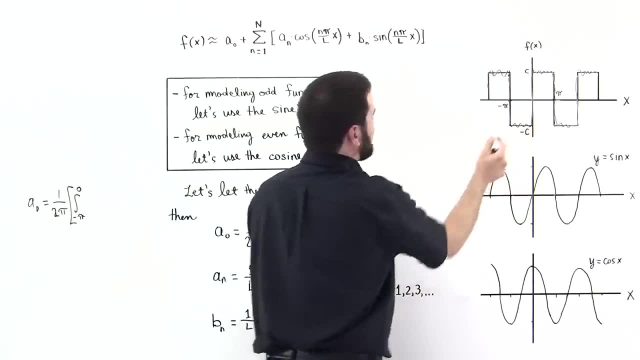 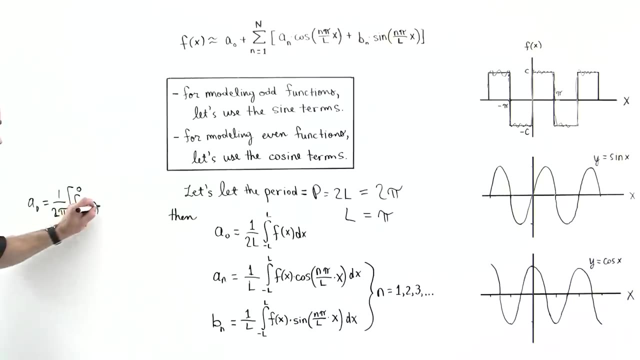 negative pi to 0, we're going to break it up. And then f of x. from here to here, f of x is equal to what Negative c? So we put f of x in here. this is negative c dx. 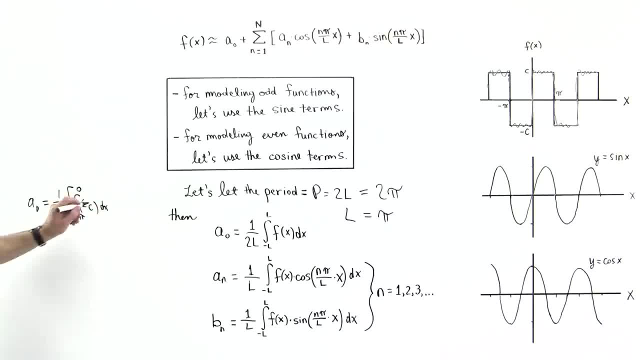 Plus from 0 to pi, and then from 0 to pi. look, the function is c. From 0 to pi, it's positive c. Okay, And if we do this, we will see that a0 is equal to 0.. 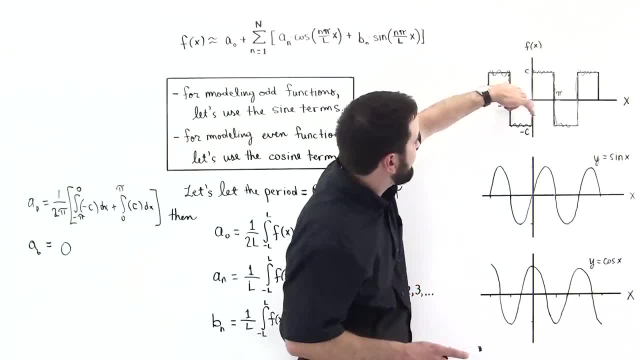 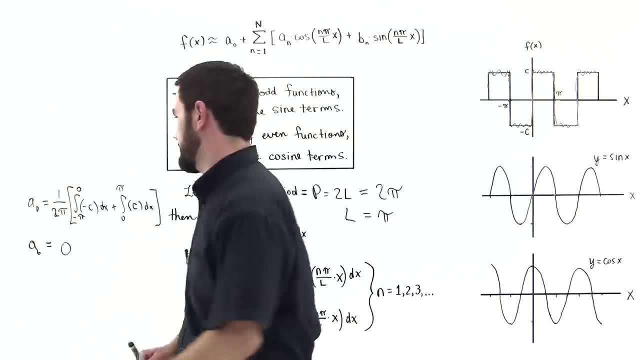 Right, Because, look at it, You have this area here which is the negative area, and you have the same area which is positive, so they cancel And a0 is going to be 0 for this example. But this is just to show you that how we're going to break this up.